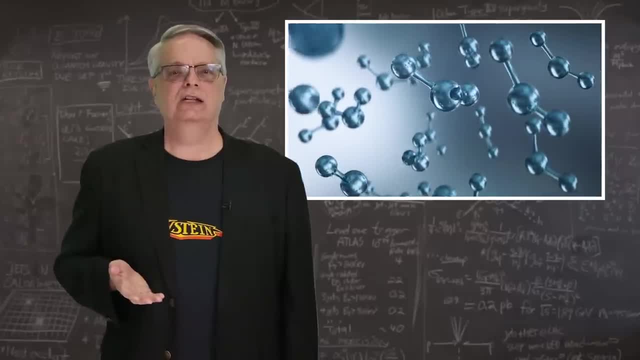 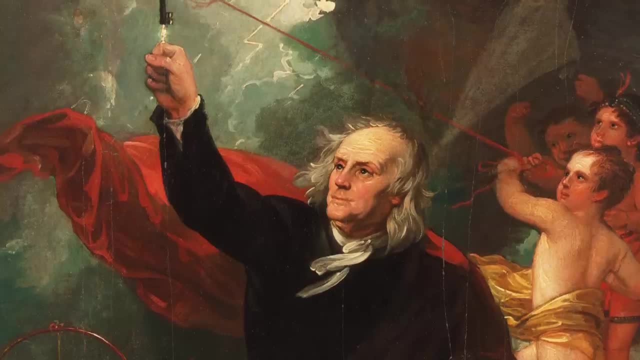 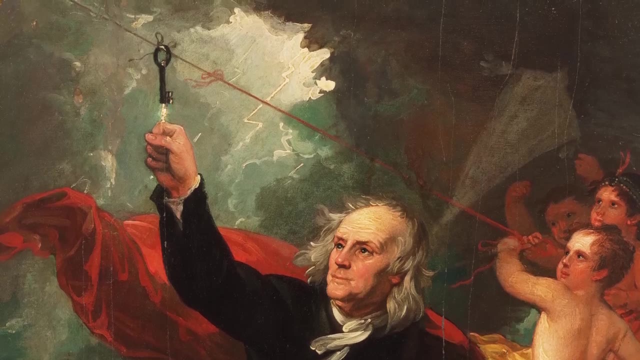 do about uncovering a deeper and more fundamental layer of nature or getting closer to understanding the underlying nature of the cosmos, they still benefit from the science. For example, back in the 1700s electricity wasn't understood all that well. It was mostly a topic for eccentric guys to putter with in their labs. 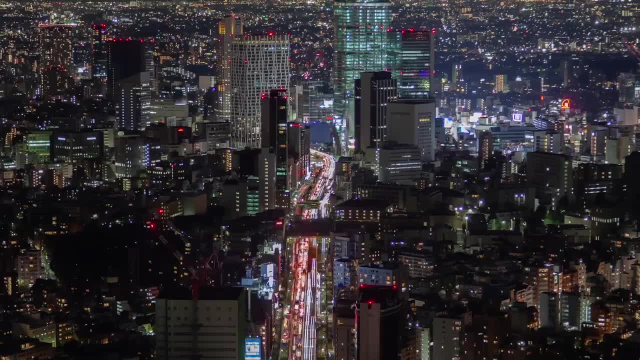 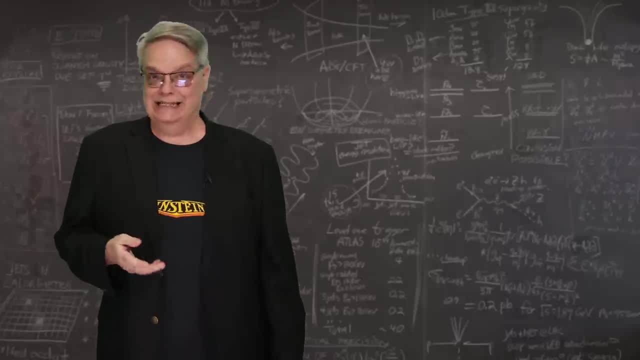 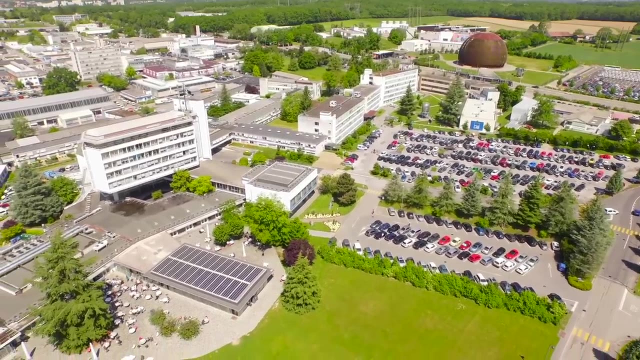 and a parlor trick used to amaze rich people at parties, And now it powers our entire society. While I personally don't understand it, particle physics isn't everybody's cup of tea. However, we've all benefited greatly from the field, For example, researchers at CERN. 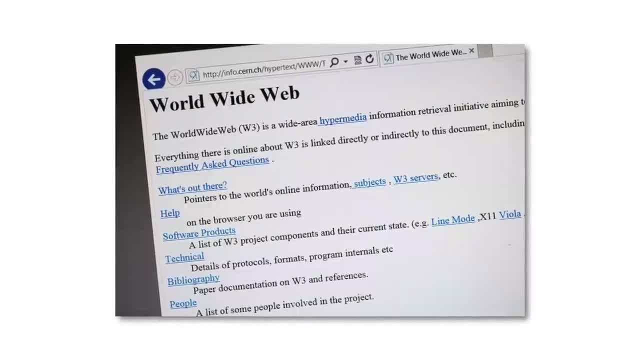 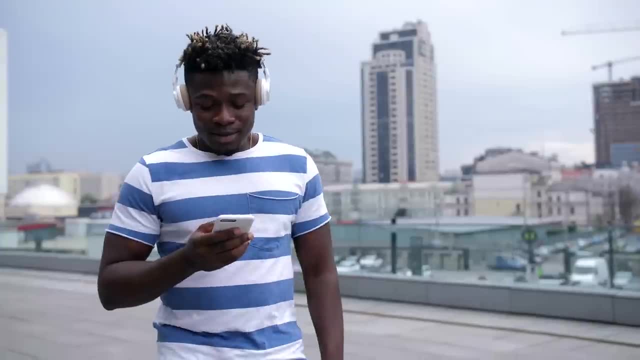 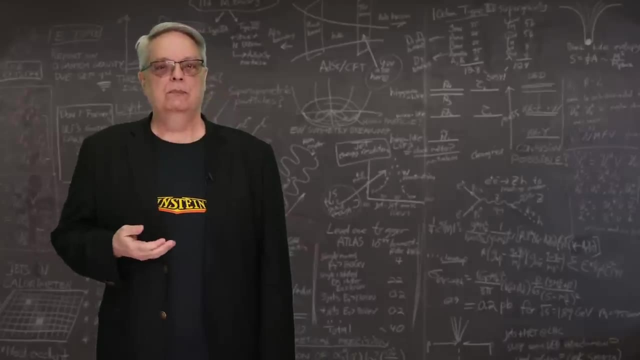 the European equivalent to Fermilab, invented the World Wide Web some 30 years ago. It revolutionized the world, speeding up commerce and communication and giving everyone with a cell phone or computer access to unprecedented information. However, for me and people like the ones who wrote the, 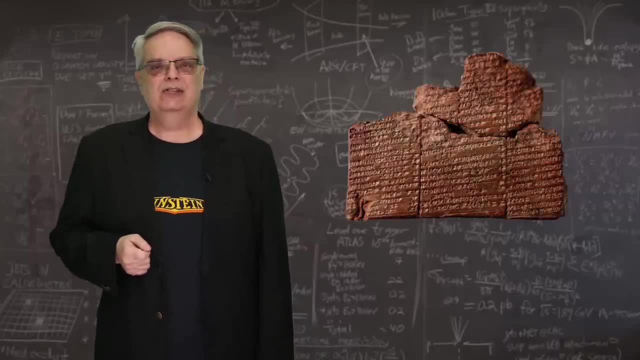 Eridu Genesis tablet over three millennia ago. these spin-offs are just nice side effects, something to make our lives easier. They don't get to the key point, which is to answer ancient questions about the universe and why we're here So fast forward until the modern day. 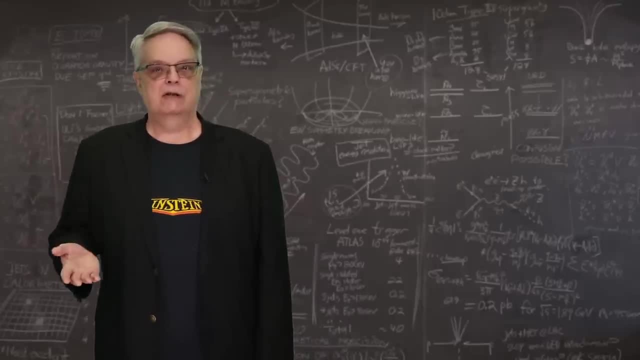 We know a great deal about the fundamental natures of matter and energy, space and time. Rather than the medieval notion of the planets moving by the beating of angels' wings, we now understand gravity and how it works. This knowledge has allowed us to explore the solar 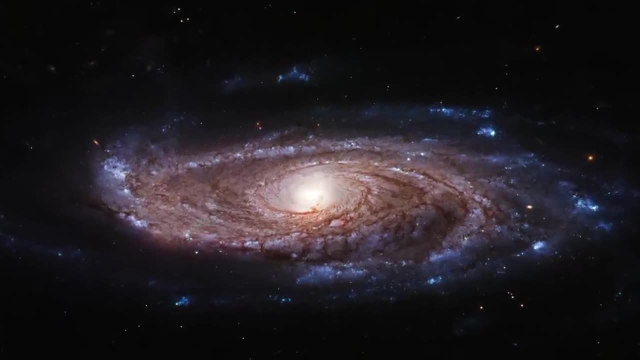 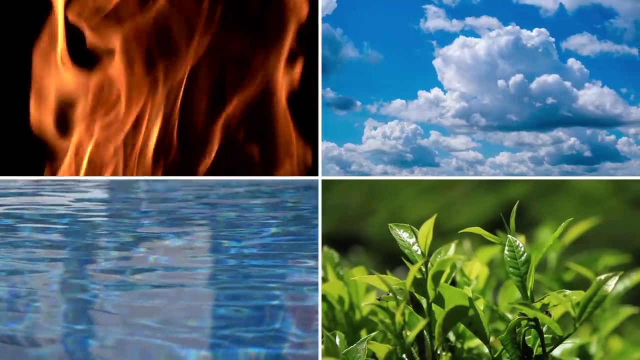 system and study the workings of galaxies and black holes. The theory that best describes the cosmos is called the General Theory of Relativity. On the microscopic side, while the ancient Greek pondered whether fire, water, earth and air were the crucial elements, 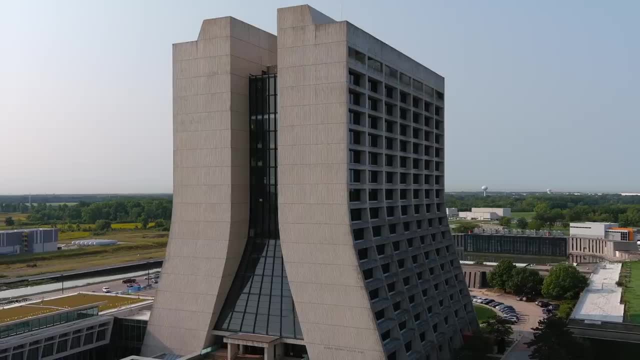 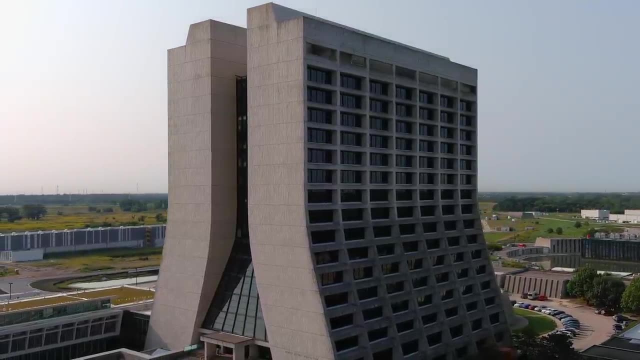 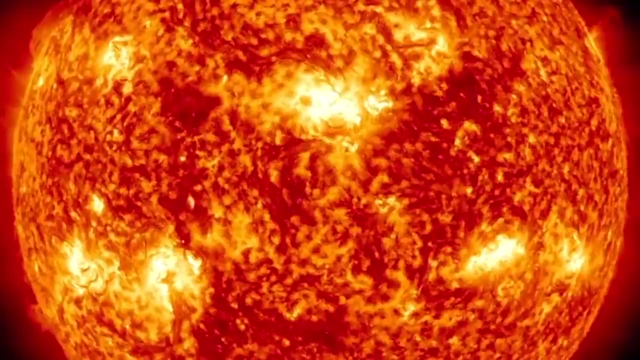 we now know of the atomic model of nature, And here at Fermilab and other similar facilities, we have dug even deeper, learning what exists inside atoms. We know of nuclear fusion, which powers the sun. We know how to transmute energy into matter and vice versa. 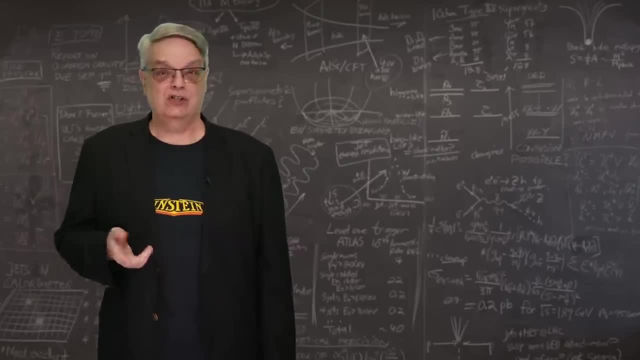 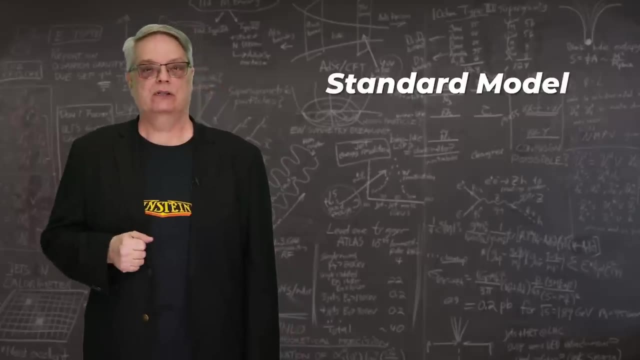 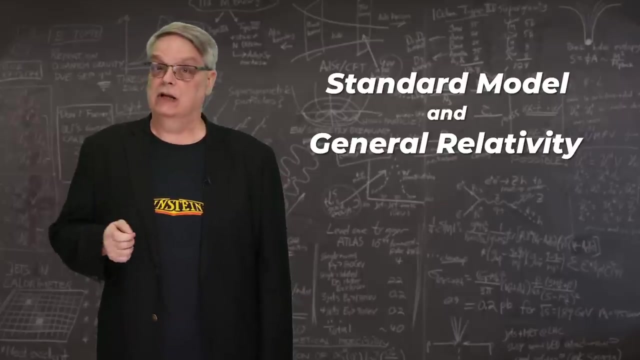 We know of a substance called antimatter, which sounds like science fiction but is definitely real. The name of the theory that best describes the subatomic realm is the Standard Model of Particle Physics. Together, general relativity and the Standard Model showcase our very best understanding of the laws of nature. We have made great strides. 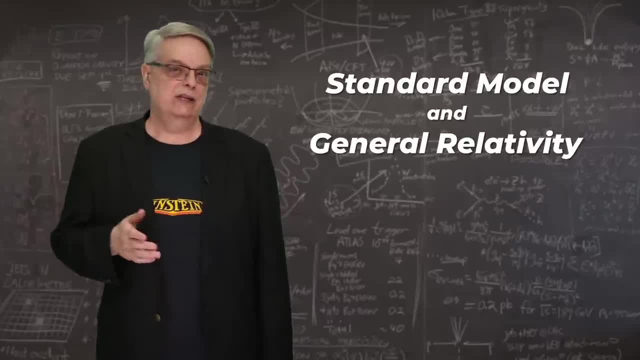 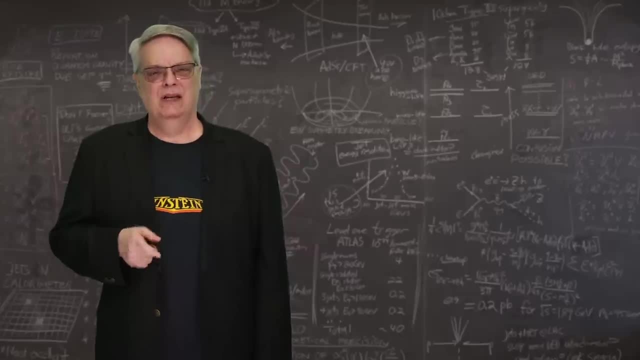 towards shedding light on the questions first written down on the Eridu Genesis tablet. However, despite our successes, we aren't done. There remain unanswered questions and I want to share half a dozen or so of them And, by the way, I've made videos going into all of my videos. 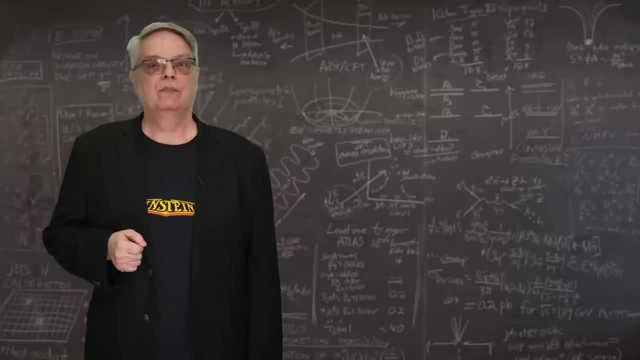 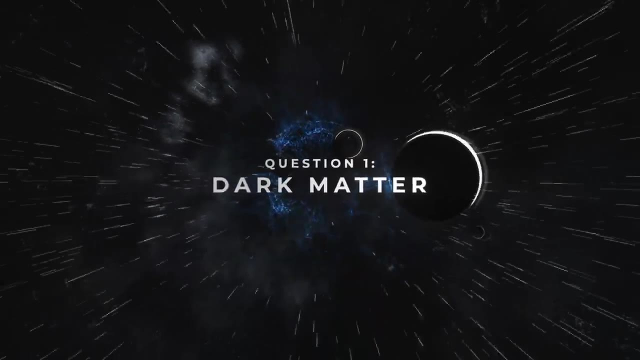 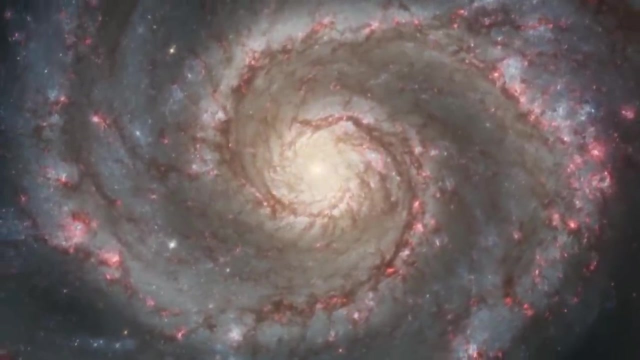 of them in more depth. The links are in the description below. My first example: Why do galaxies rotate much faster than the known laws of physics allow? One possible explanation is that there exists a form of matter called dark matter and that exerts a gravitational force but neither emits nor absorbs light. 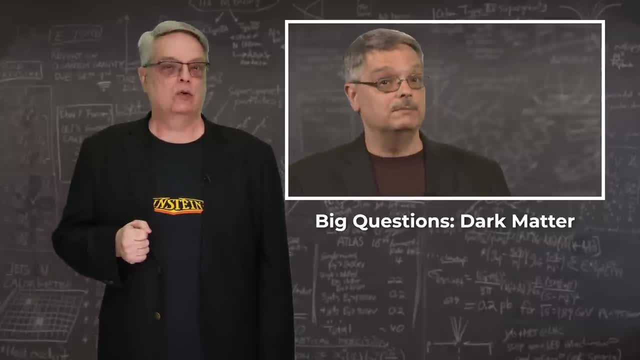 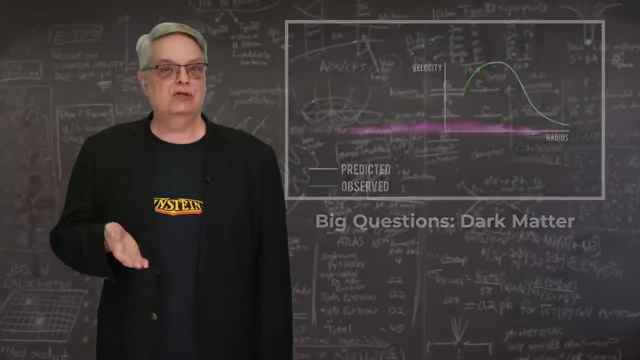 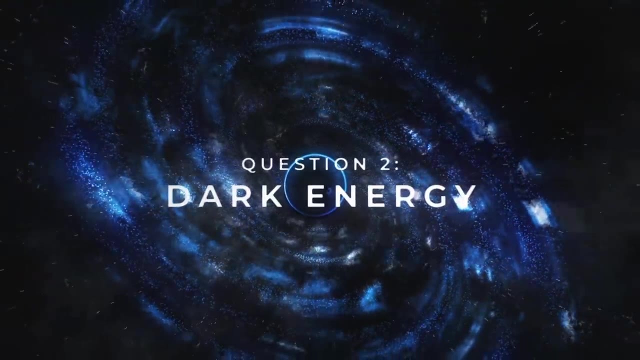 Whether dark matter may or may not exist, finding the answer to the question of the speedily spinning galaxies remains. Scientists around the world are seeking to find the answer using various experimental approaches and comparing theoretical predictions to measurements. Here's another example: The universe is expanding, which the theory of the Big Bang. 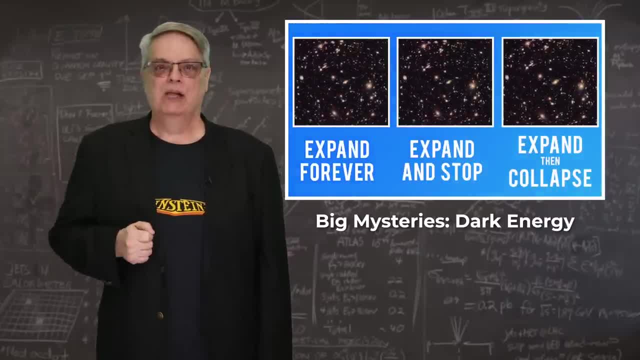 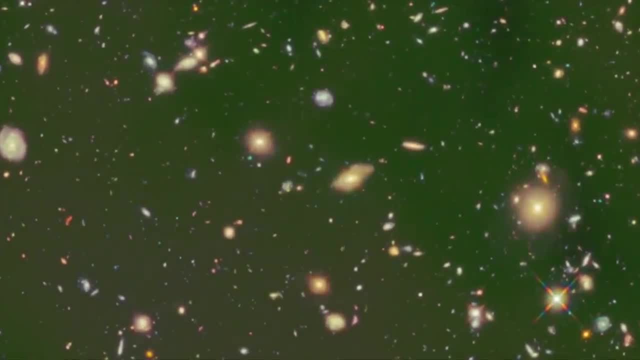 explains. However, the expansion is accelerating, requiring that there be a form of repulsive gravity. The proposed solution for this is called dark energy. However, we don't really understand why We don't understand dark energy, except to think it's a property of space. 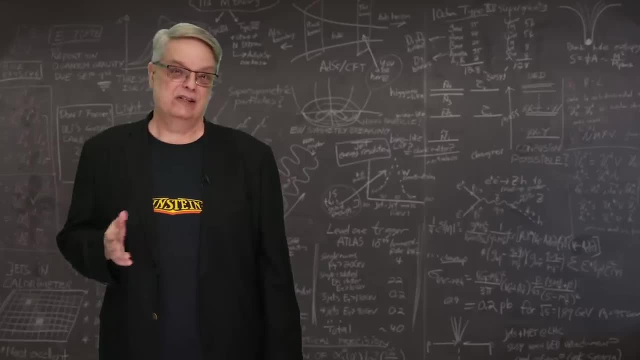 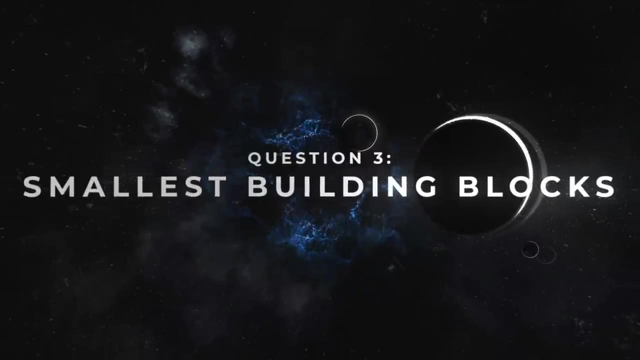 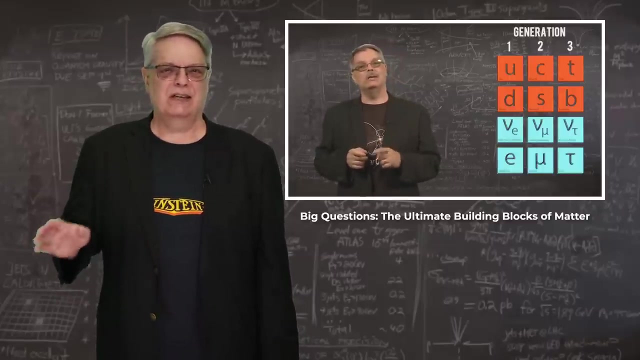 The full explanation eludes us, and a detailed understanding of the accelerating expansion of the universe remains an open question. We also know that there are interesting regularities in the patterns of quarks and leptons. While it just might be a coincidence, the pattern looks a bit like the chemical periodic table. 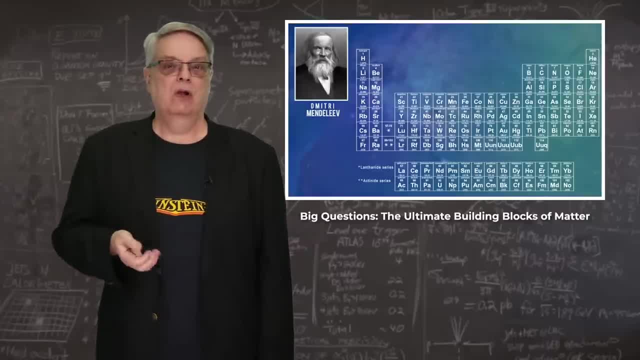 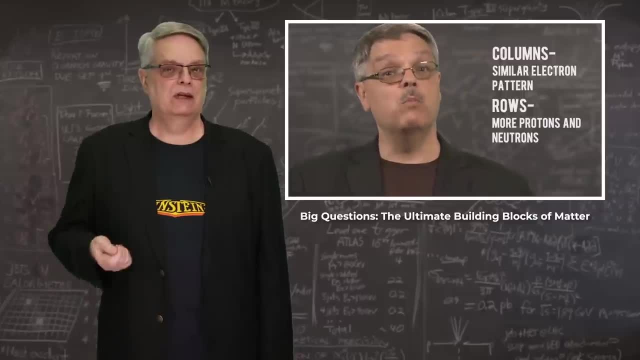 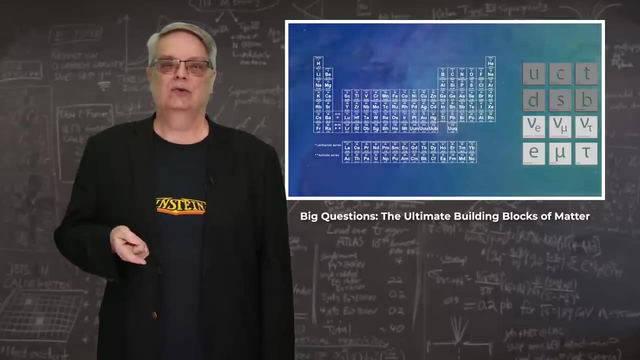 of elements. The explanation for the periodic table was that atoms were made of smaller things arranged in complex ways, with a nucleus and an electron cloud. The patterns in quarks and leptons may or may not have the same answer, But whether or not that's true we still don't know. 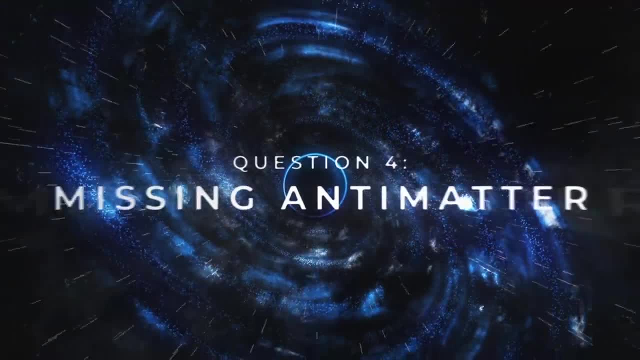 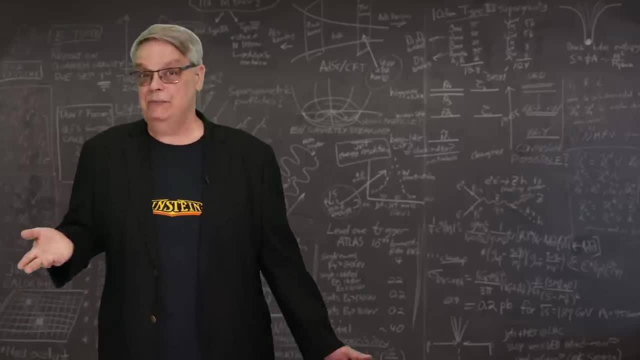 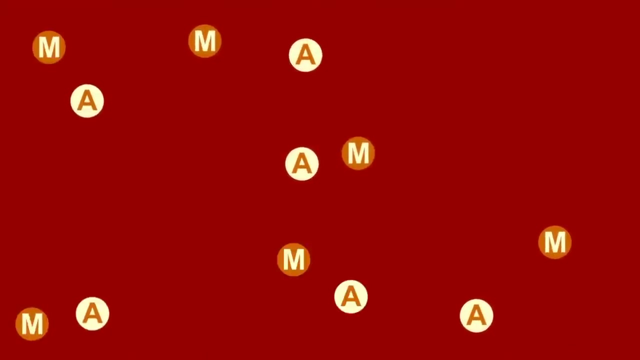 the answer of why the pattern exists. My fourth example involves understanding the nature of the origins of the universe, which relies on two seemingly contradictory things. One is that the universe began in a hot, dense state called the Big Bang, and the early universe was full of energy. 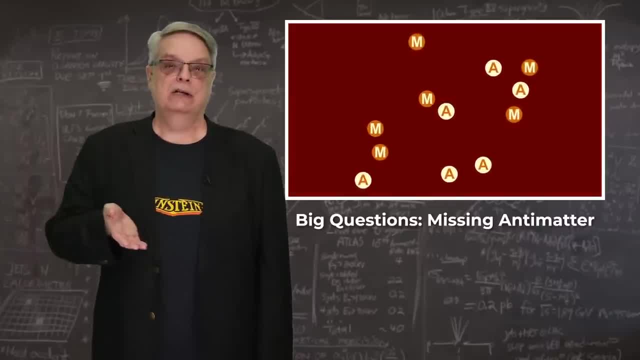 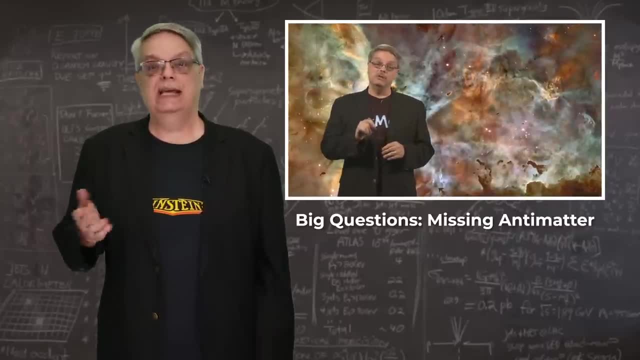 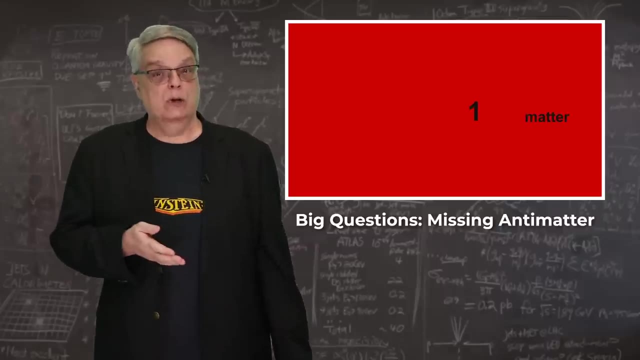 The second thing is that energy can be converted into matter and antimatter. Both of these things have been validated, Yet when we combine these two ideas, we find that we can't explain our universe. Our universe is made solely of matter, while the theories say that we should have equal 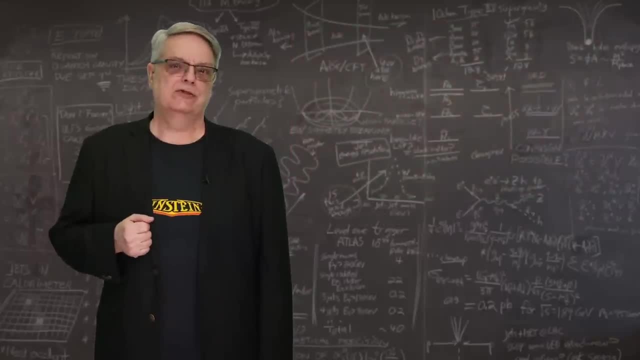 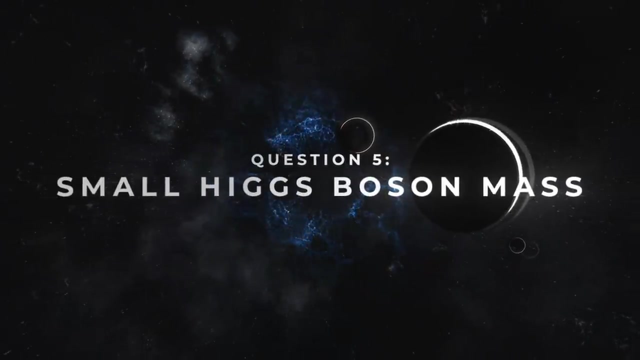 amounts of matter and antimatter? That's another unanswered question. In fact, it's one of the driving reasons why the Fermilab research program is upgrading our particle accelerator complex and developing huge new particle detectors. The discovery of the Higgs boson was the culmination of half a century of work. The Higgs boson. 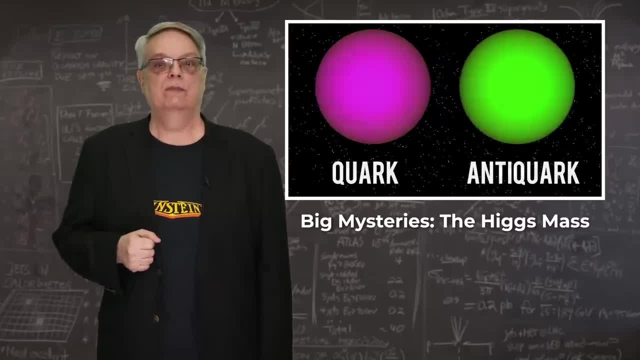 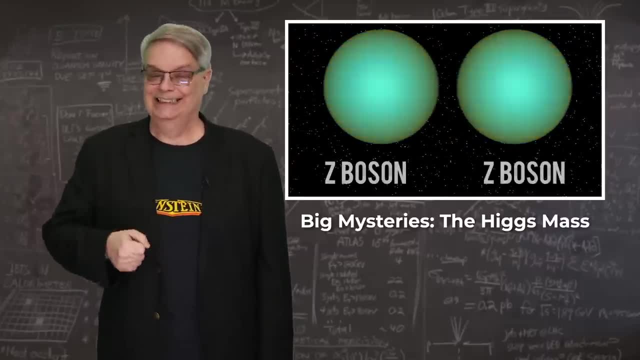 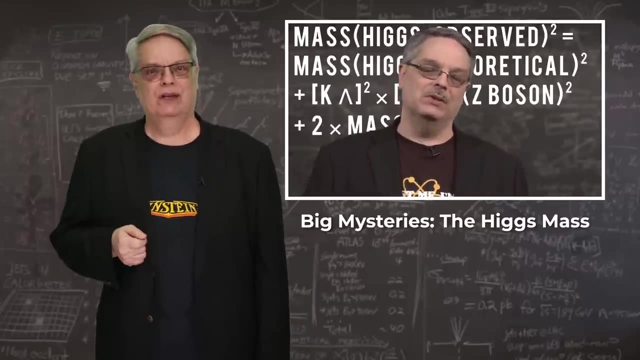 was predicted in 1964 and discovered in 2012.. The boson gives mass to subatomic particles. It was predicted and we found it. However, there is a problem. The standard model predicts that the mass of the Higgs boson should be ginormous, but it's not. While we have some, 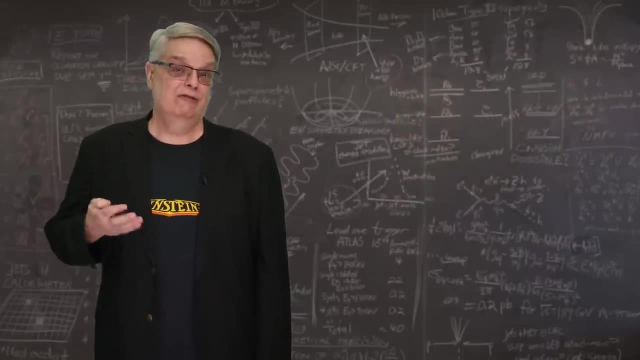 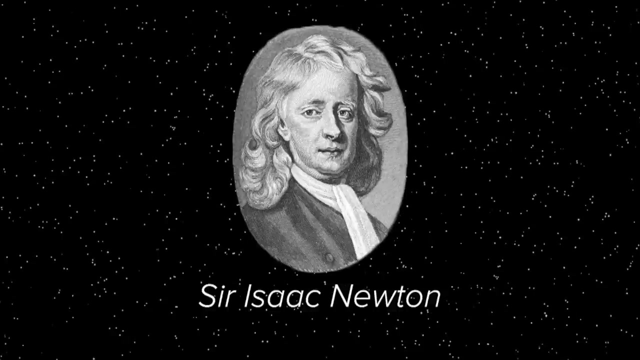 ideas as to why prediction could be flawed. we have a fifth unanswered question. This is a technical point, but it shows that, as successful as the Standard Model is, its answers are incomplete. The sixth question has to do with a historical trend. Isaac Newton realized that the gravity on Earth and in the heavens are one and the same. 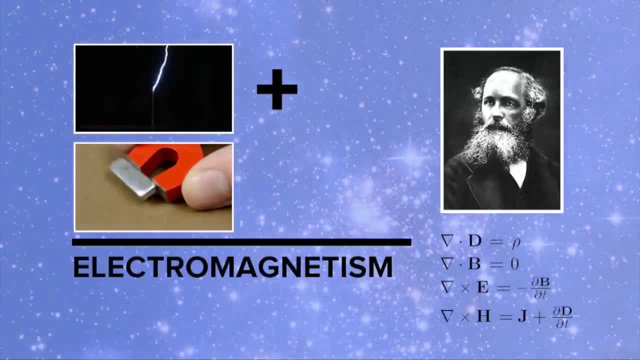 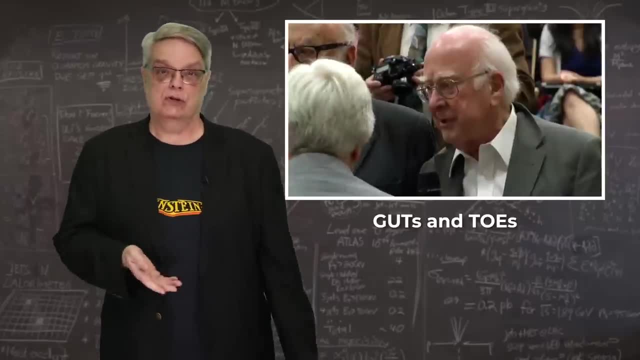 James Clerk Maxwell proved that electricity and magnetism are the same, And with the discovery of the Higgs Boson, researchers proved that electromagnetism and the weak nuclear force are the same. It remains quite possible that in the future we'll discover additional cases of seemingly 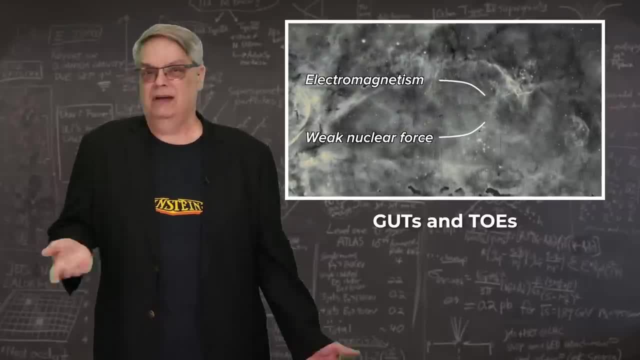 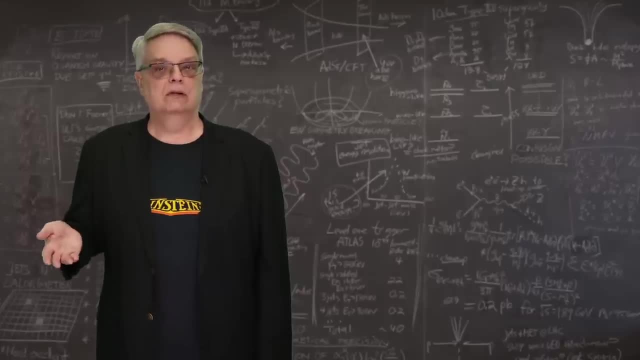 different forces actually having a single cause? Maybe at the base of it there's only one force. It's another question that, if we answer it, will teach us something fundamental about the laws of nature. I listed half a dozen questions, but there are more. 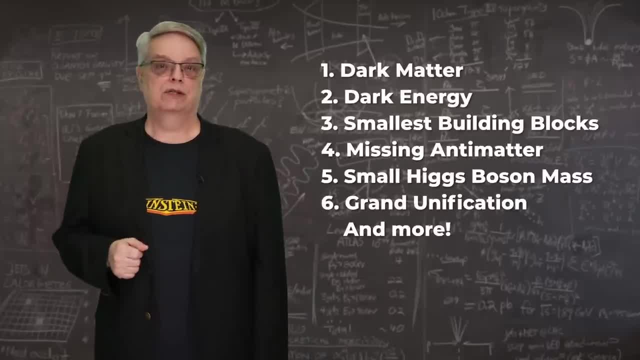 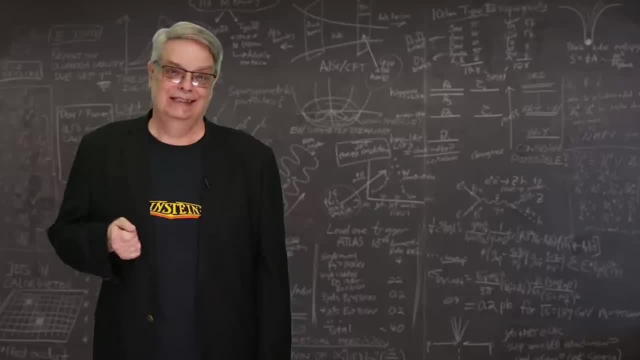 While the Standard Model and General Relativity are amazing accomplishments, they aren't complete. They leave questions that we need to answer to get to the bottom of things. So that brings us to the related question, which is: how do we answer these science questions? 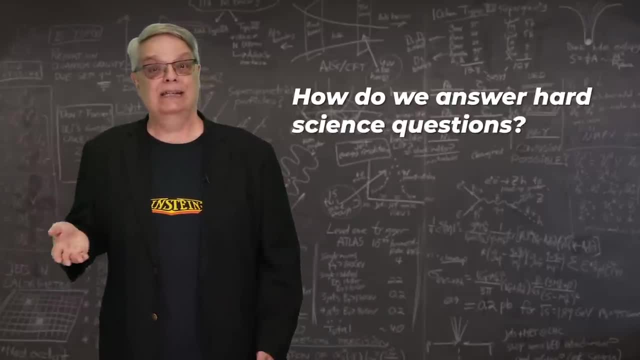 And that answer is simple. We have smart people think up ideas, and we have other smart people think about ways to build equipment that can both test those ideas and generate data that will point researchers in the right direction. The problem, of course, is that nobody knows the answer. 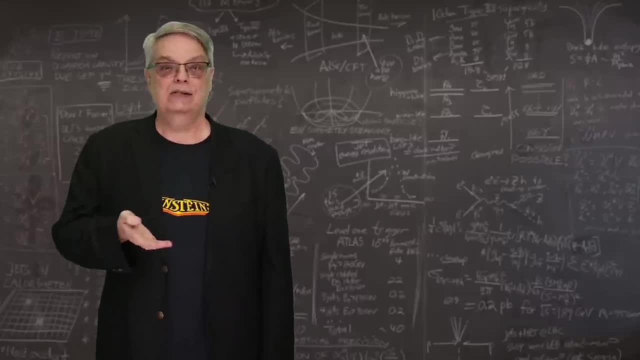 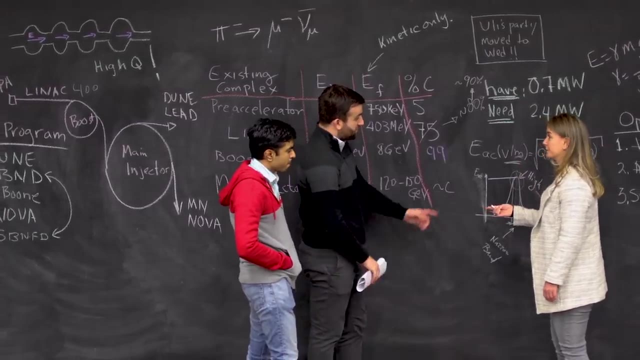 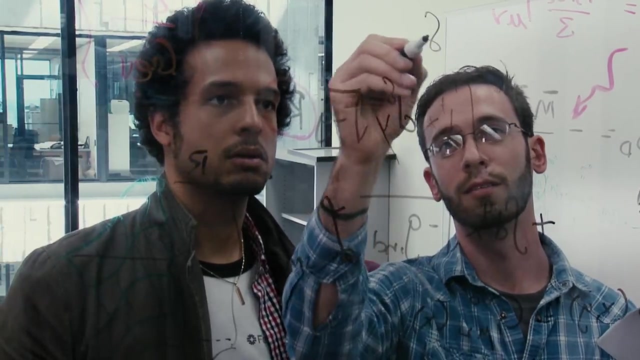 So what we have to do is tackle the questions in different ways and come up with many smart ideas. We test those ideas against existing data and throw out the ones that disagree with past and current measurements. What is left are theories that agree with everything we know and potentially answer. 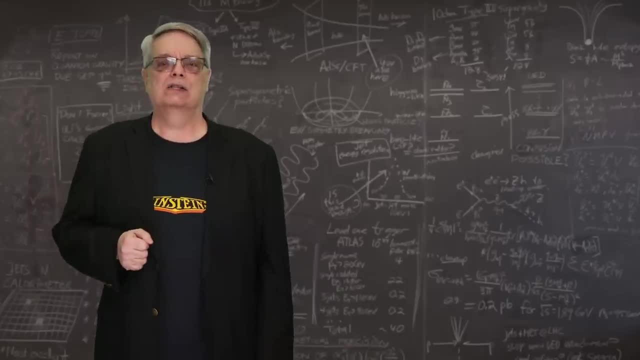 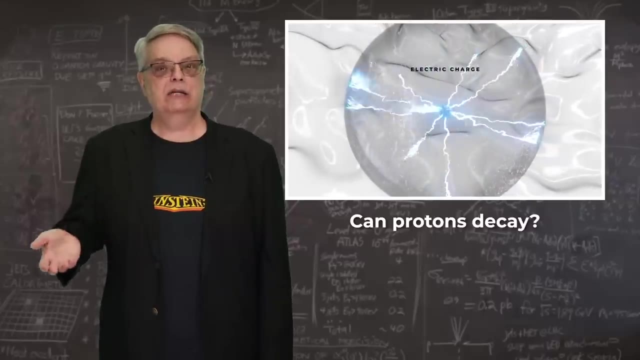 unanswered questions. How does this work in practice? Well, as an example, let me return to my video on proton decay. Back in the 1980's, some theoretical physicists came up with some ideas that might explain how the various forces might unify. 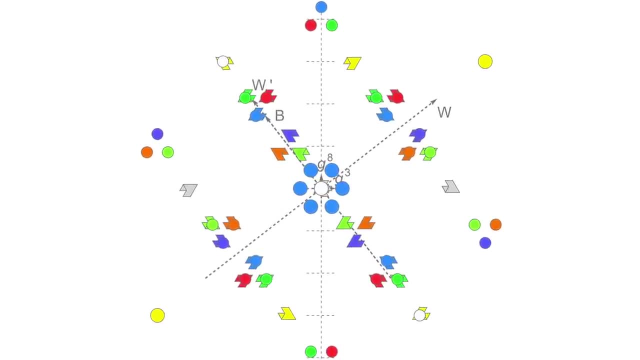 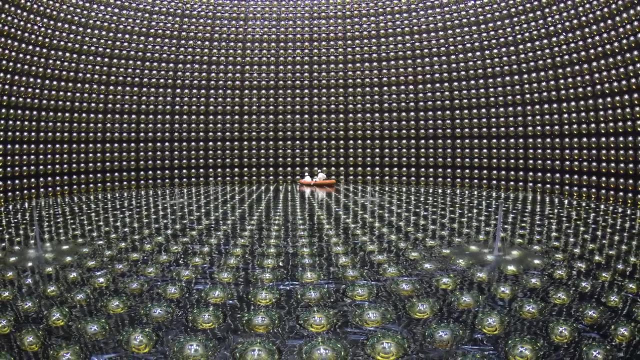 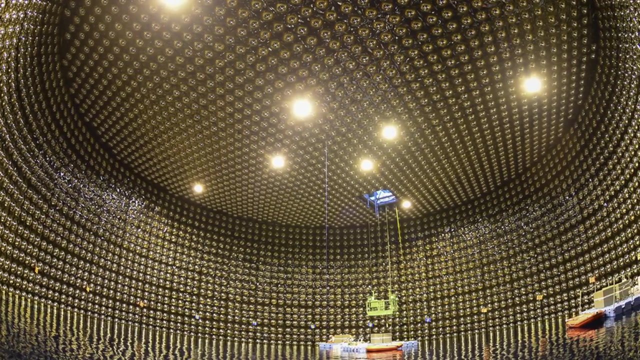 The mathematical ideas were complex, involving a lot of geometry, But one consequence of these ideas was that protons would decay, So giant detectors were built to study the stability of protons. The result was that no proton decay was observed, But the detectors did observe solar neutrinos and neutrino oscillations. And the result was that no proton decay was observed. Nobel prizes were awarded for these discoveries. Moving forward, researchers wouldn't build a detector just to look for proton decay. However, if detectors were built for other reasons, that were big enough, it would be. 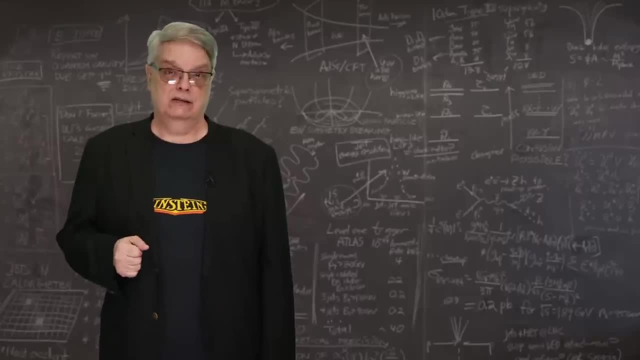 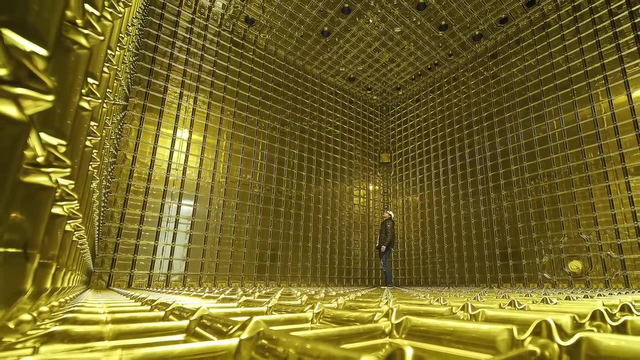 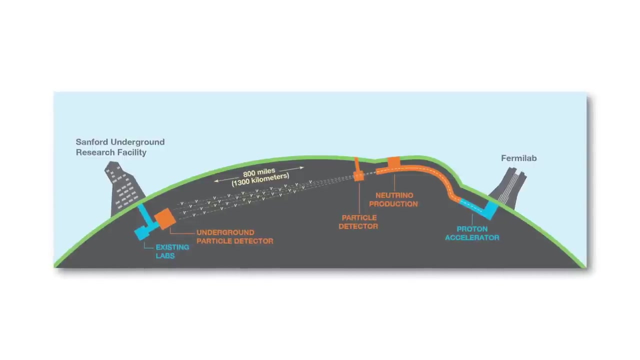 irresponsible to not also use them to look for proton decay in other elusive subatomic phenomena. That's the case with the Fermilab Deep Underground Neutrino Experiment in Japan's Hyper-Kamiokande. They are both being built to do neutrino studies and proton decay studies come more or less. 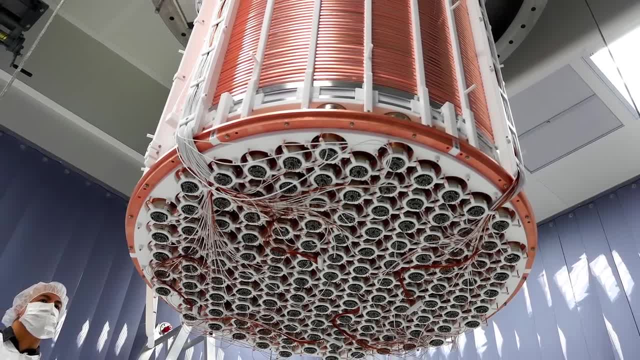 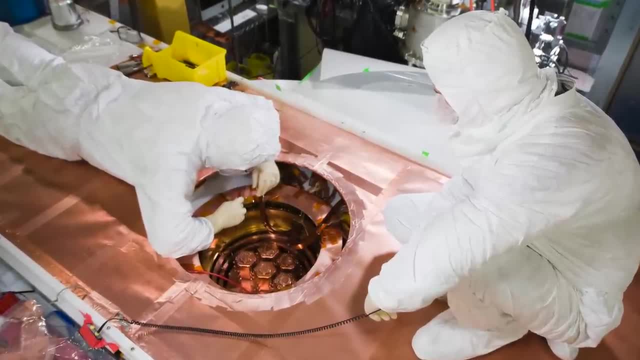 for free. On the dark matter front, there have been dozens of experiments looking for lots of different kinds of dark matter, and none of them have found it. So while it could be true that this means that dark matter doesn't exist, it's still. 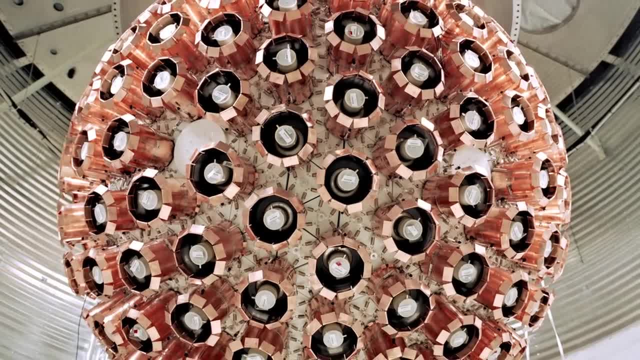 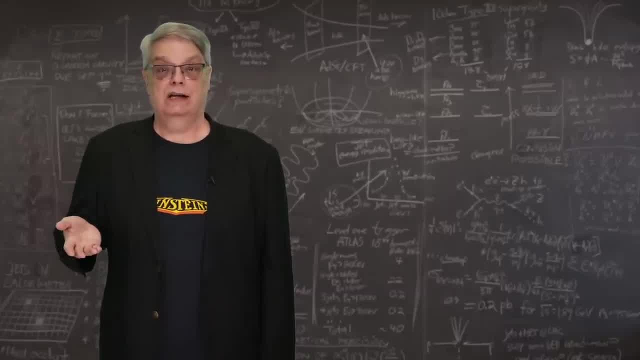 true that the question of why galaxies rotate so quickly remains unanswered. Because of that, scientists continue to come up with ideas, some of which involve dark matter And some of which explore other explanations. Whatever the explanation, we'll only be able to resolve the question using experiments. 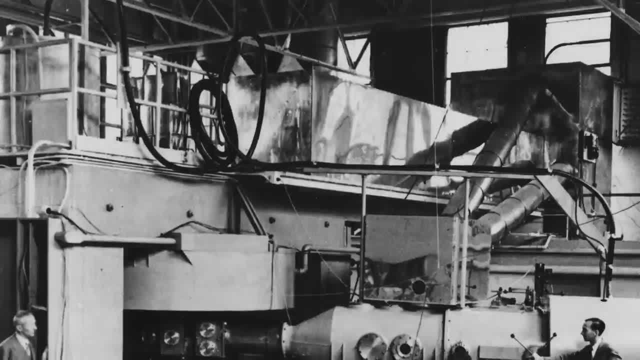 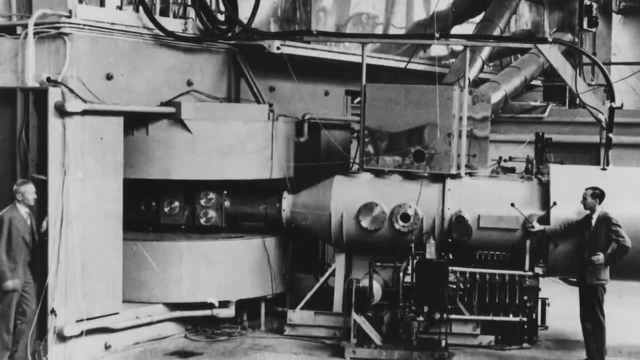 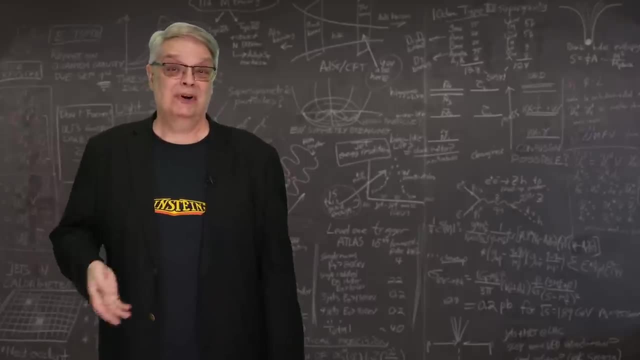 and data. Then there are particle accelerators. Since their invention about 100 years ago, particle accelerators have been an incredible source of data for physics research Indeed. without particle accelerators, the Standard Model would have never been devised. We would have never known about quarks. 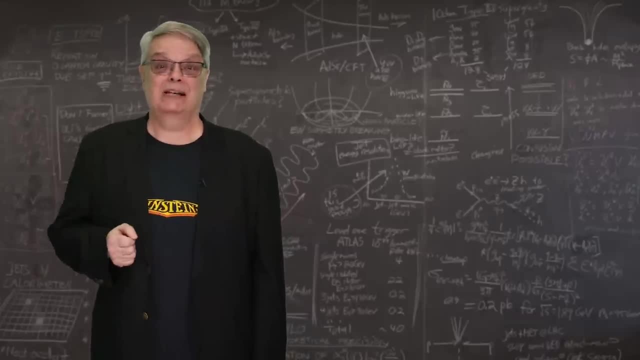 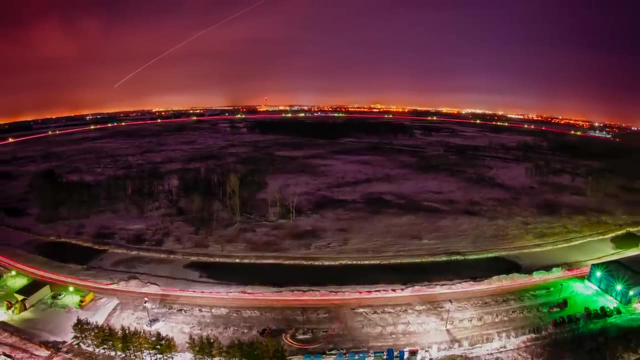 We would have never understood the Higgs boson And how particles get mass. We'd be stuck back at the understanding of a century ago. Fermilab's Tevatron was the world's most powerful accelerator, from the mid-1980s until. 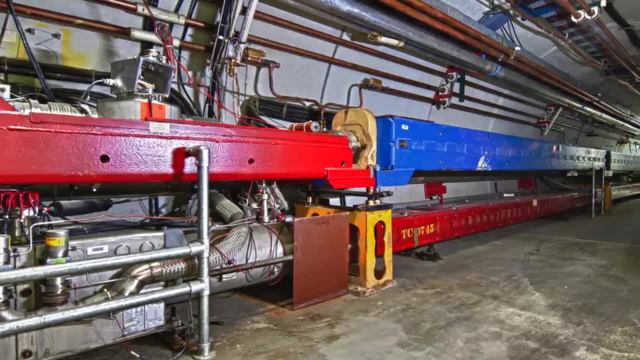 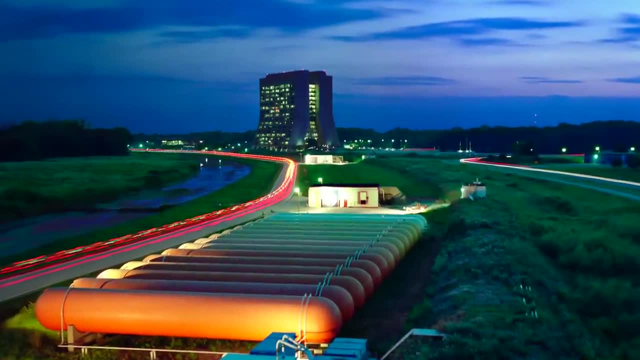 2009.. During that time, Fermilab researchers discovered the Tau neutrino and the top quark, made important measurements that might help us understand why there is no antimatter in the universe, and made many other advances in understanding the subatomic world. 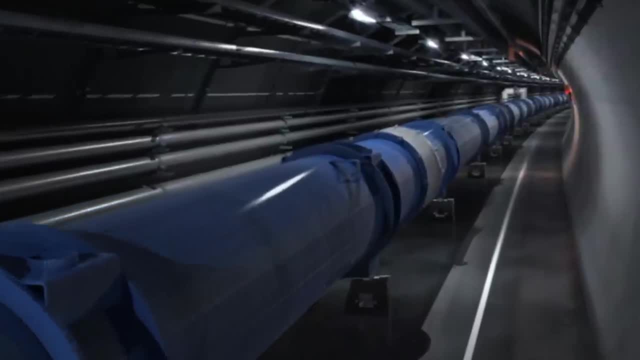 Currently, the Large Hadron Cluster is the largest hadron cluster in the universe. It is the largest hadron cluster in the universe. It is the largest hadron cluster in the universe. The Large Hadron Collider is the most powerful accelerator. Using it, we have discovered the Higgs boson and we are exploring in more and more detail. 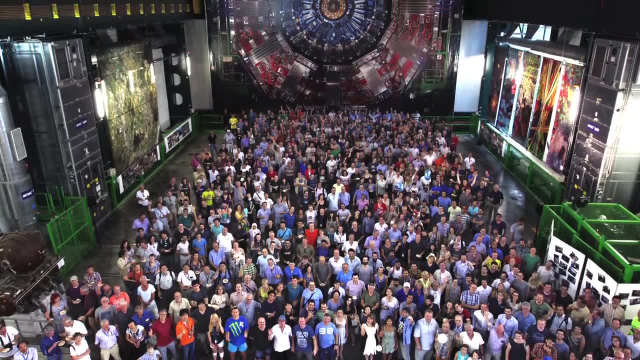 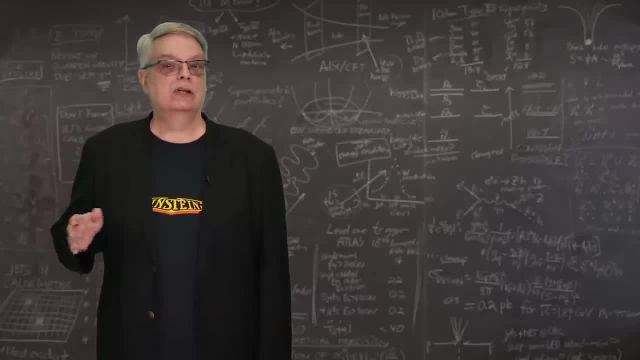 how the Higgs boson interacts with other bosons and quarks. We've also found many particles made of quarks that had never been seen before. Combining all of the measurements done using the accelerator, we've published more than 3,000 scientific papers to share the data and knowledge we've gained. 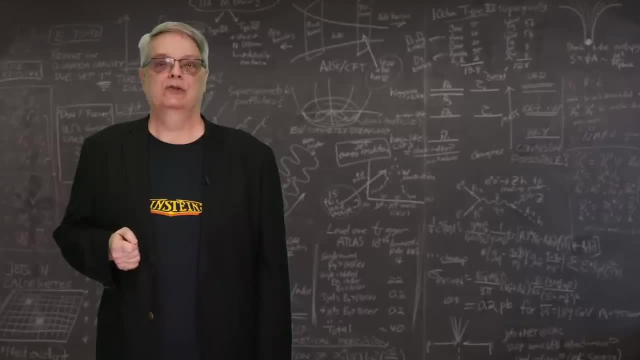 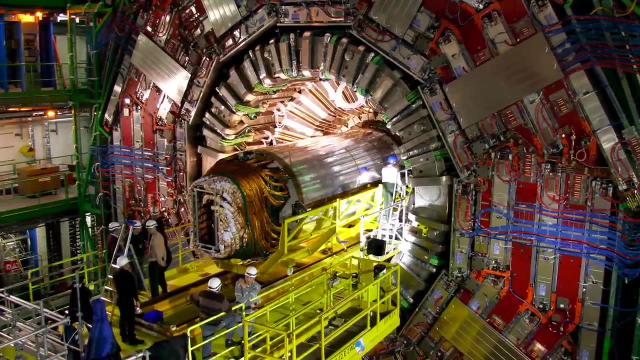 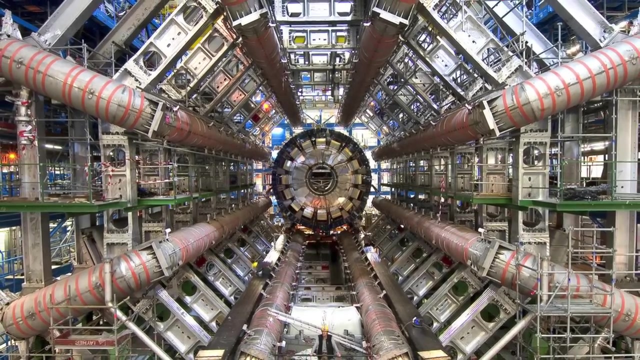 Despite these discoveries, we still have many unanswered questions, And even the next generation of experiments are unlikely to answer them all. Based on the century-long success that we've had with building more and more powerful accelerators, it's very reasonable to think that finding more answers requires a more powerful particle. 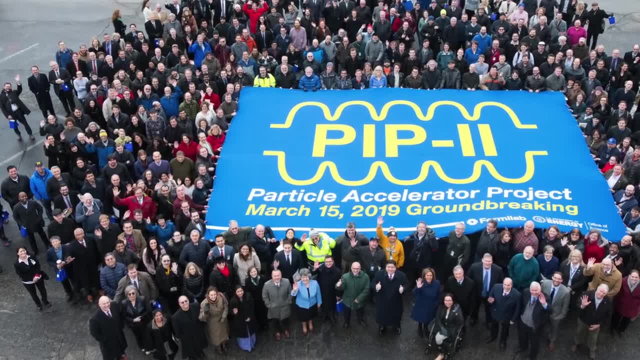 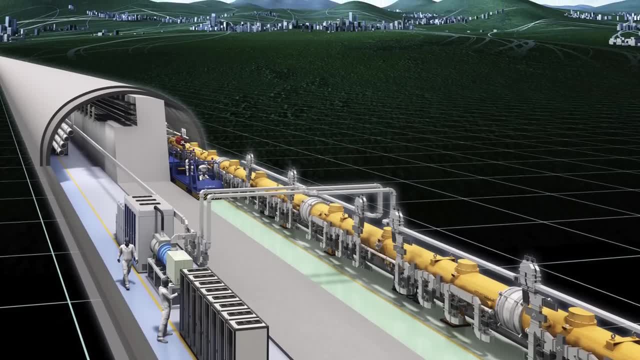 accelerator. Of course, it's important that when we build such an accelerator and the associated detectors, that they be multi-purpose machines that can answer many questions Basically. that way, you get more bang for your buck. I think a key point is that it's important to think about how we can build more powerful. 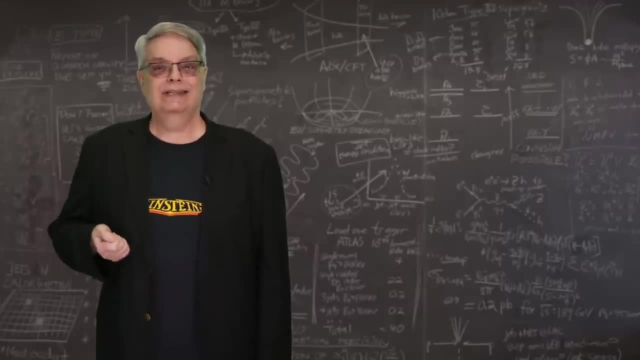 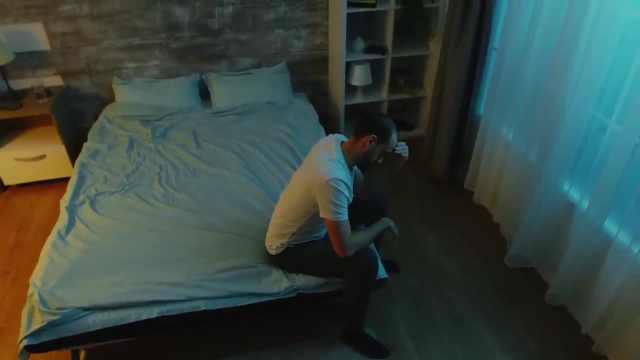 accelerators, And it's important to remember that the equipment isn't what's driving this. What's driving the inquiry are the questions, the unanswered conundrums that are keeping us awake at night To answer questions. sometimes bigger is better. 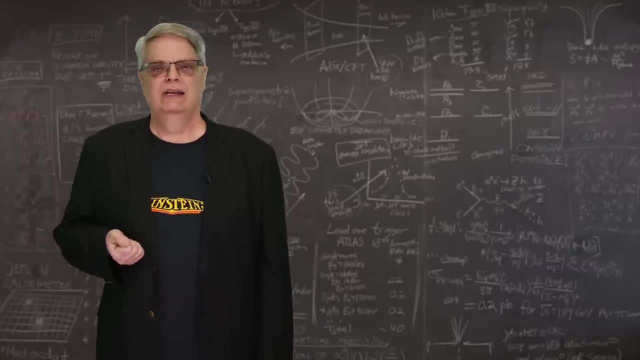 On the other hand, sometimes a small experiment fits the bill, And it takes careful thought to decide what's best. In order to recommend which proposed experiments are the most promising ones, the particle physics community gets together every five or ten days to discuss the most promising. 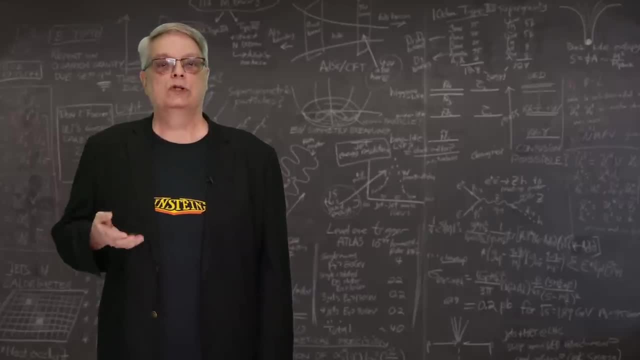 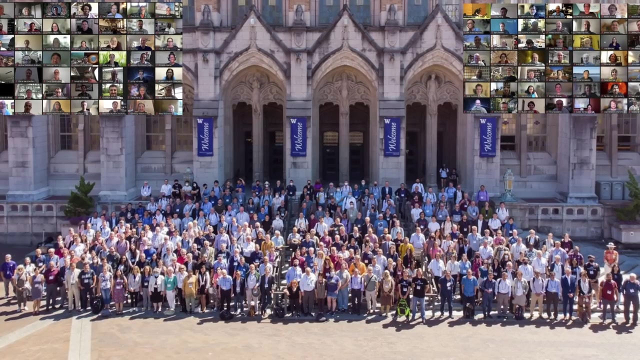 ones. It takes five or ten years to take stock and decide which approaches are more likely to generate results. The European scientific community just finished such a review, while the American evaluation is going on right now. For several years, using what is called a SNOMAS process, researchers have examined 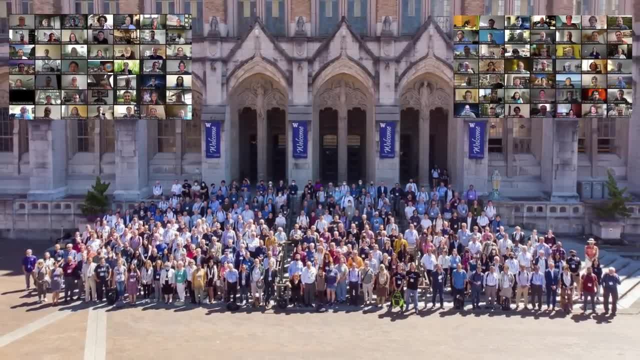 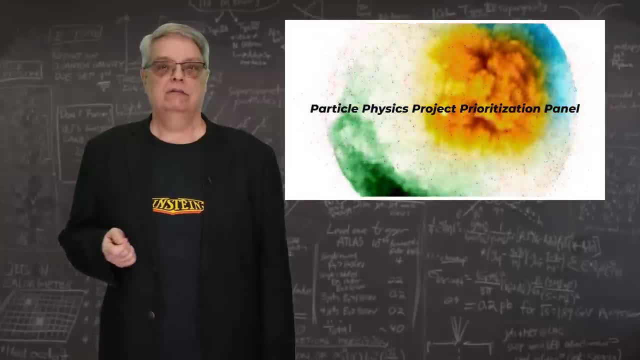 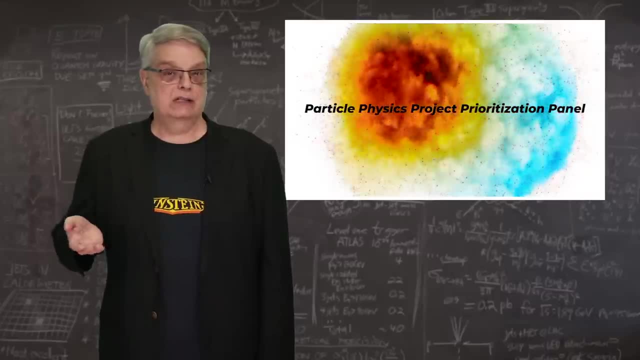 many ideas to make a case for this future project or that, And now a group called the Particle Physics Projects Prioritization Panel- or P5, is evaluating all those ideas. P5 will then do its best to emphasize the promising ideas and reject the ones that seem. 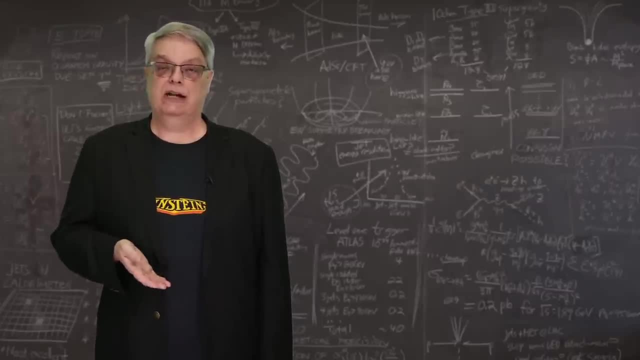 less likely to help. Finally, P5 will make their findings available to funding agencies, which will make the final determination on which projects to pursue and which ones not. It's a process designed to select the most promising future research. But as you think about what scientists are doing, it's important to go full circle. 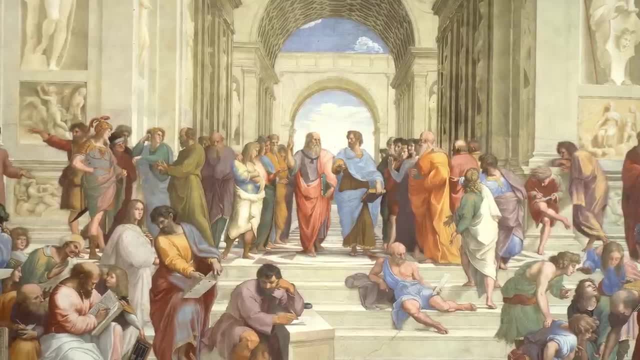 and remember why we're doing this at all. Just as the first step of the research process is to determine which projects are most promising, we need to think about the next steps, When the first writings wrestle with questions like the origins of the universe and the deepest. 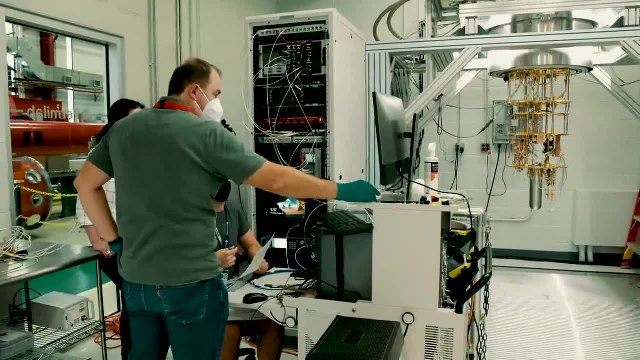 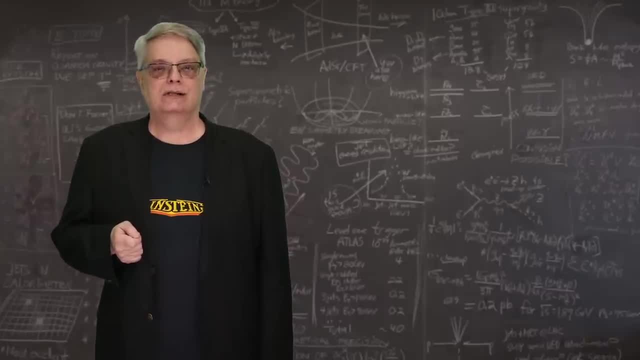 laws of nature. scientists today do the same thing. We've made incredible progress over the past few centuries, but the journey continues. The final answer eludes us, and it's going to take a lot of hard work and clever experiments to get us to the end of the road. 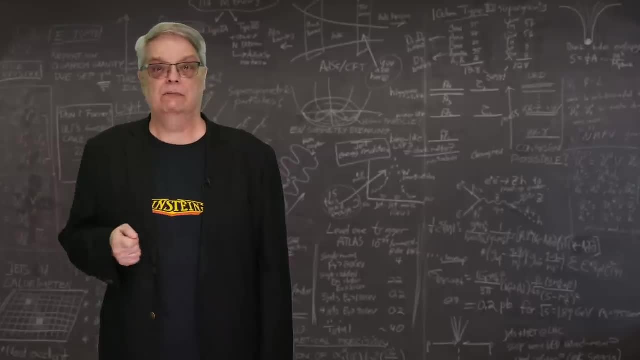 This isn't a project that will be solved in months or years. It will take lifetimes. It's important to remember an inescapable truth: The only way to complete a journey is to go full circle. The only way to complete a journey is to keep taking steps. 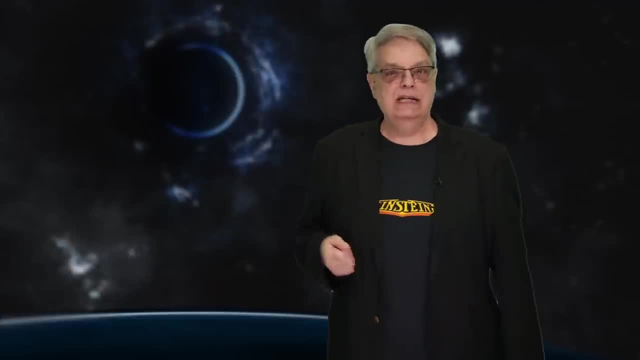 And that's what we're doing. OK, that was maybe a deep video. Every so often it's important to take a step back and see the big picture. This neat problem may be interesting, or that one may teach us something, But at some level. those are all details. 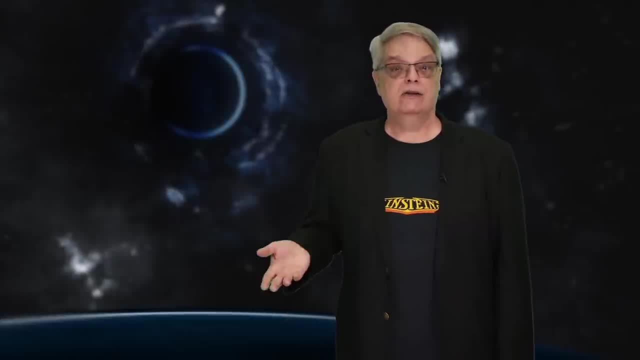 The final answer is much bigger than any question. On the other hand, progress depends crucially on answering questions, and answering questions depends on having the right equipment and experiments to do that. Only by this hard work will we maybe finally shed light on the biggest questions ever tackled. 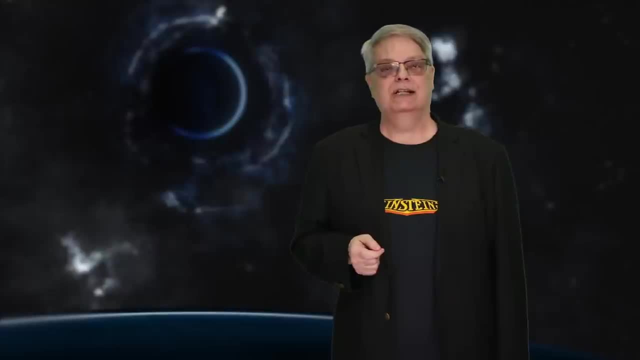 by humanity, Well, physics ones at least. And that will be a great day because, well, as I've often said, physics is everything.